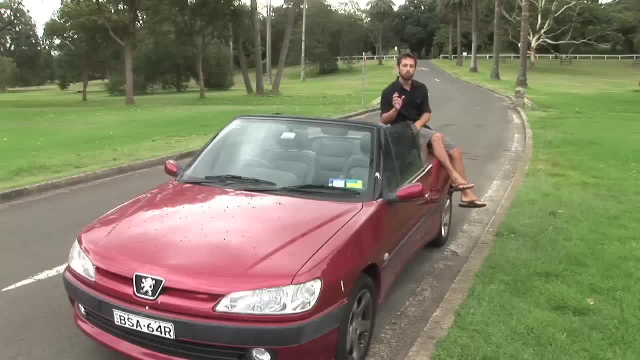 all the same, But there's an important distinction between the terms mass and weight. Mass refers to the amount of matter in an object, whereas weight is a force. It's the gravitational attraction that the object feels towards, in this case, the Earth's center. So I've 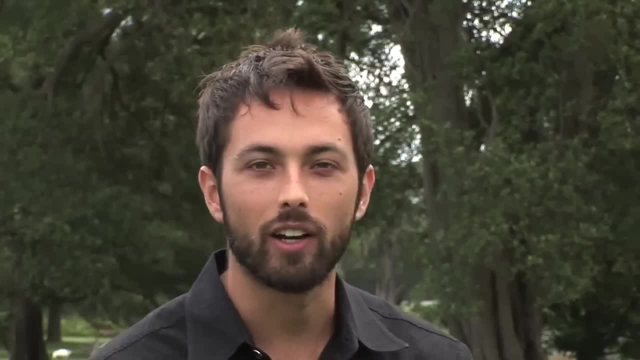 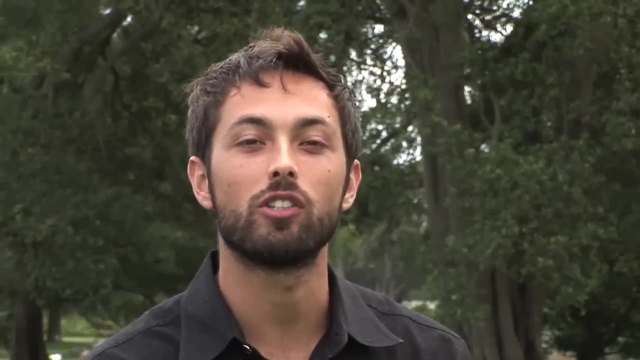 got a little experiment today where I brought my car out here. I'm going to ask some people why is it difficult to push my car? And my bet is their answer will be because the car is heavy, Because it's heavy, Because you're in a spaceship. 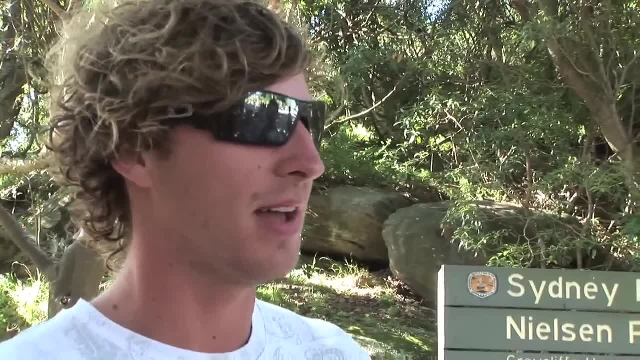 It's so heavy. It's heavy. It depends if it's uphill or downhill. It depends if it's uphill or downhill, but the car's heavy. A big rock, you would think would be heavy. Anything that's big, you would think would. 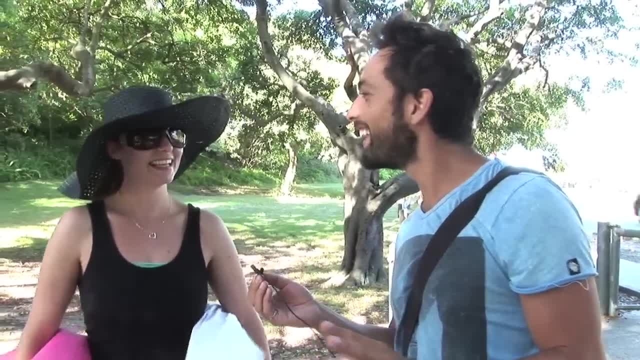 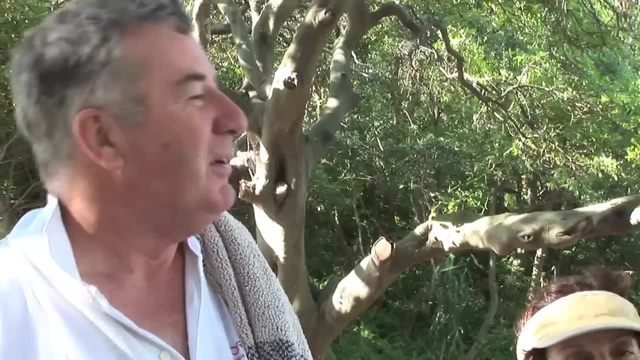 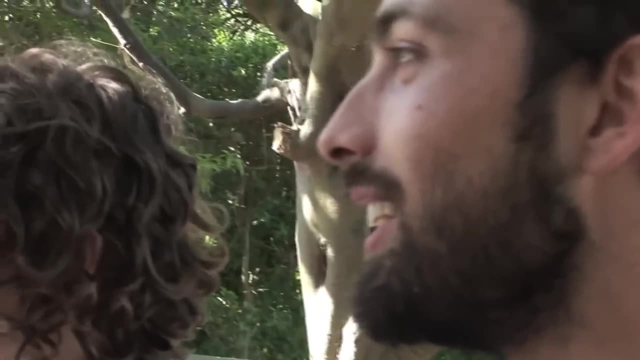 be heavy. It's too heavy, It's heavy. yeah, Oh, it's a bit lighter than I thought It's got its weight. Weight is responsible. What is weight? Weight is mass in a gravity. What is this gravity thing? 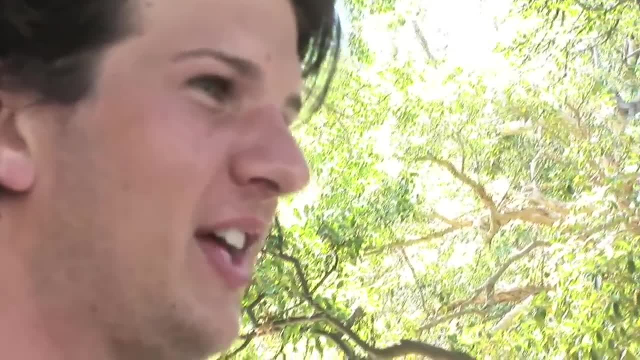 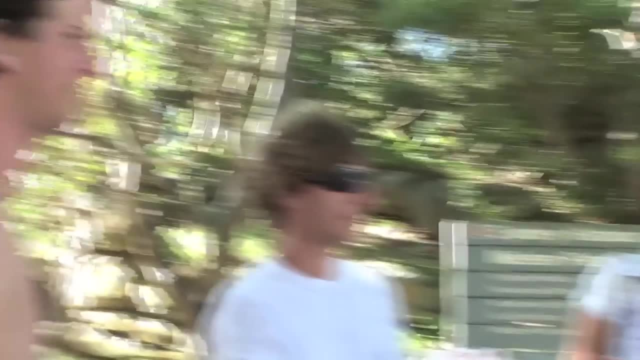 Gravity is what keeps the core of the Earth. Your car is pulled towards the center of the Earth, Yes, So if you push it, let's say you're pushing your car, you're not pushing it up. do you know what I mean? 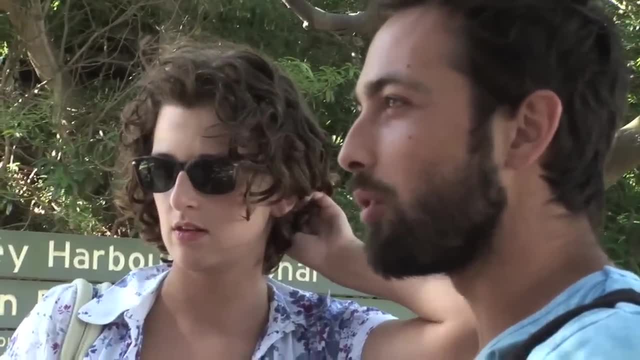 No, But it's still hard to push. Yeah, So do you think weight's responsible for making it hard to push? Well, it is weight. I mean, like you know, the lighter the car, the easier it is to push. 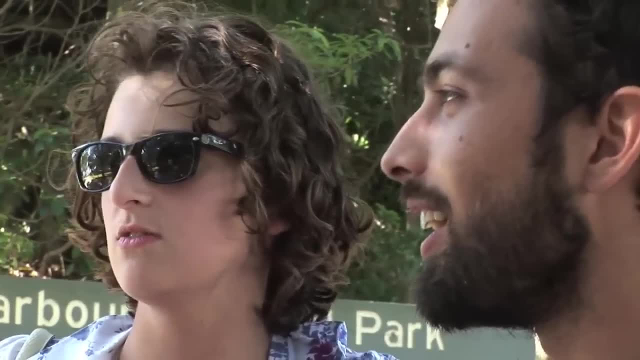 So yeah, Like weight only exists because of gravity on the mat, Because weight and gravitation. But I'm not trying to lift the car right, I'm just trying to push it. That's a really good question. Do you have like a huge, like big rock you would think would be heavy, Anything that's. 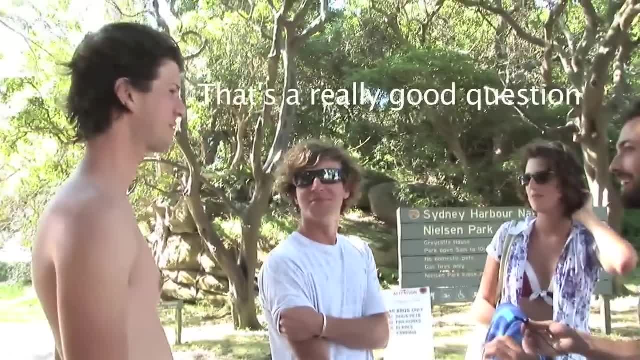 big you would think would be heavy, So a car, but I'm not lifting it, I'm pushing it. so it's the gravity over there. Yeah, But this is my question, right? Yeah, yeah, But I'm not trying to lift it. 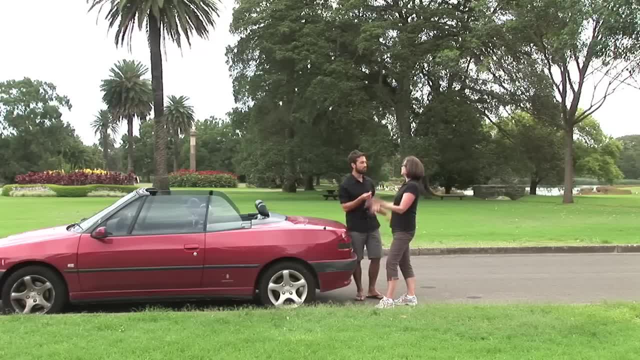 No, that's true, Pushing it, But it's still hard to push. So why is that? Because, like, if I lift it, I understand you saying it's heavy. It would be heavy, yeah, And then it would be really hard, But we're pushing it and we're actually getting it. 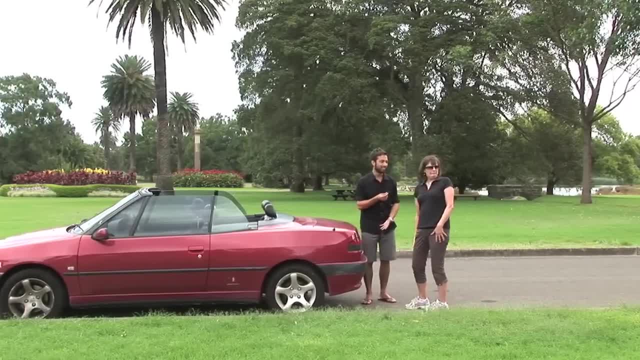 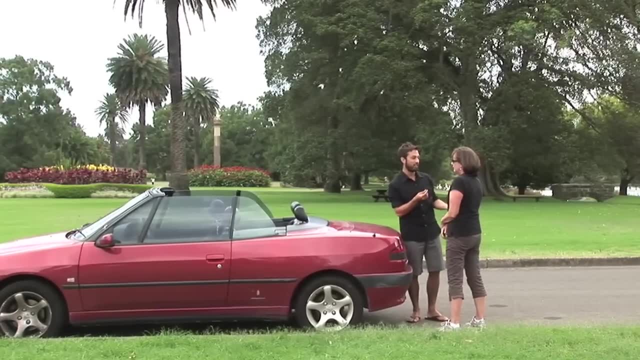